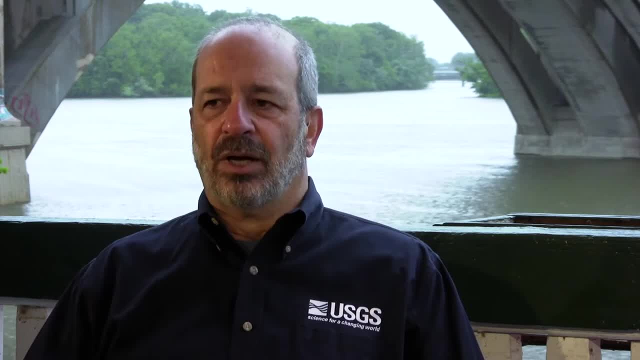 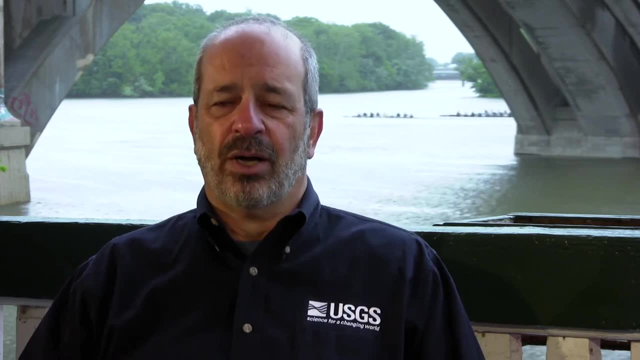 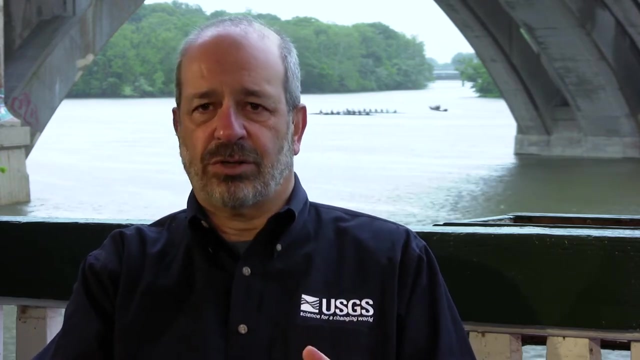 Are we making progress? Are we making progress? Are the goals of the Clean Water Act being met? And we said we have a very difficult time answering that question because we're not set up to answer that in a broad national context. So the confluence of seeing internally how difficult it was to answer these questions. 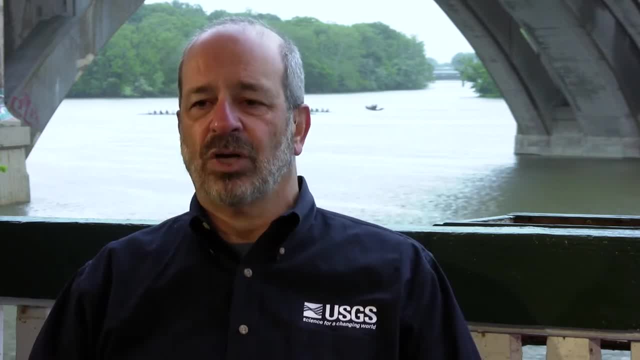 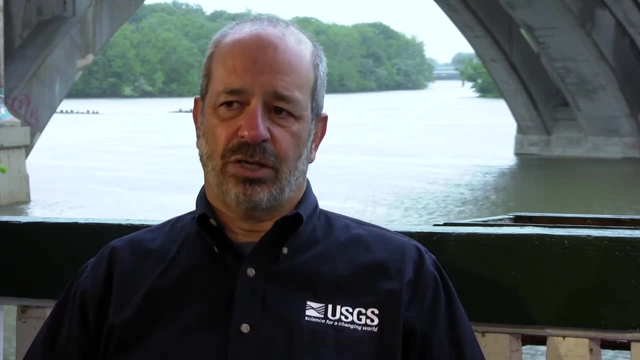 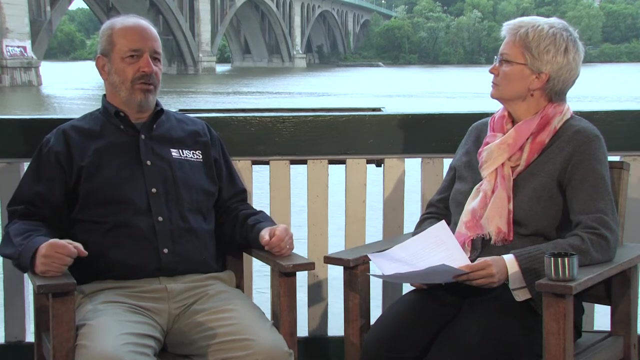 and being asked externally by members of Congress. we got to thinking we need a program, we need an organized, structured way to try to answer these kinds of questions. We created an internal team chaired by Dr Jacob Rubin of our Menlo Park California research group. 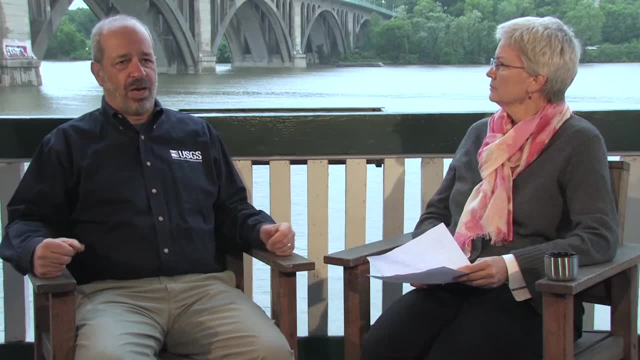 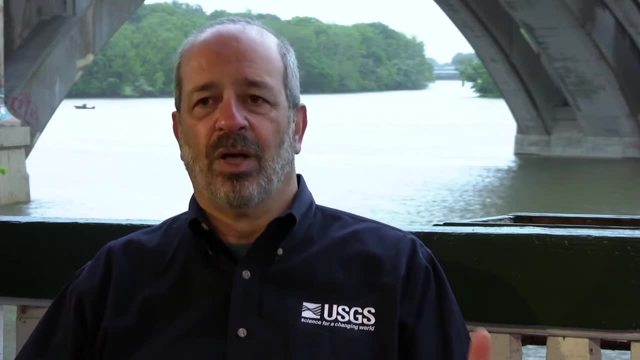 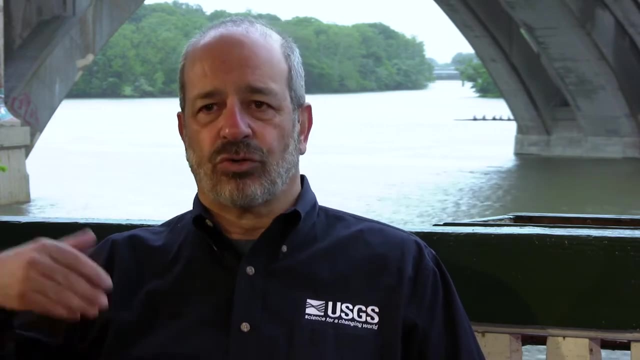 and I was fortunate enough to be among the five people that was on that committee that conceptualized how to do a national water quality assessment program, And during the mid-'80s we designed that. Then we spent several years in a pilot effort trying out the concepts that we had laid out. 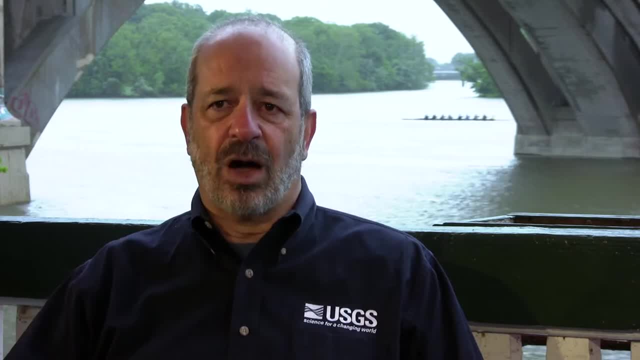 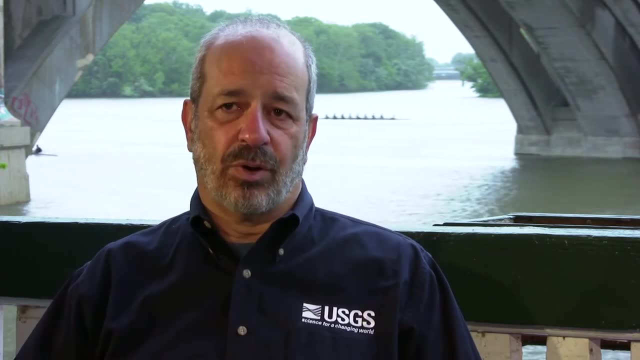 and then we really got the green light from the Congress in the late 1980s to begin this program. And so we're now a little over 20 years into that program and it's been a thrill for me to see the success of that program. 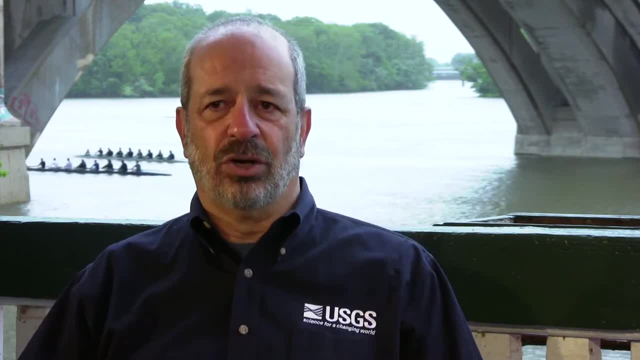 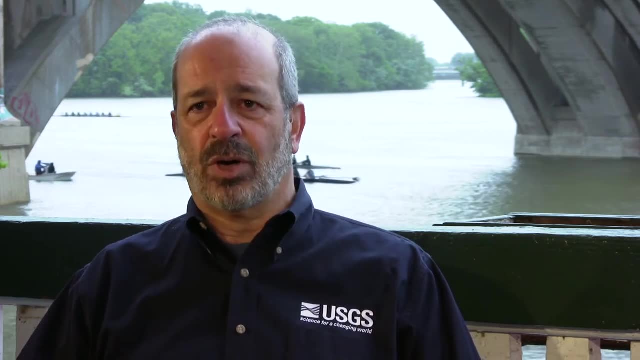 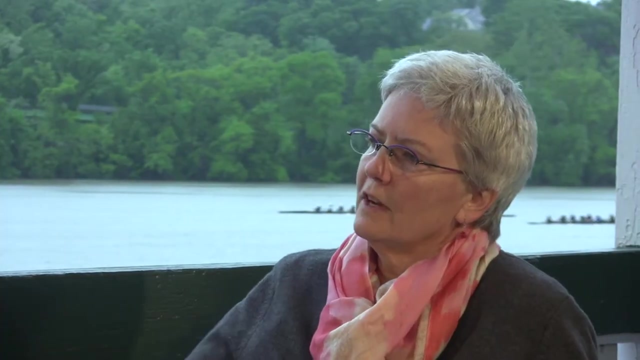 and that kind of a national organized effort coming to fruition and answering not all the questions, but many very important questions about our nation's water quality. What are some of the most exciting and useful parts of NAWQA, the National Water Quality Assessment? 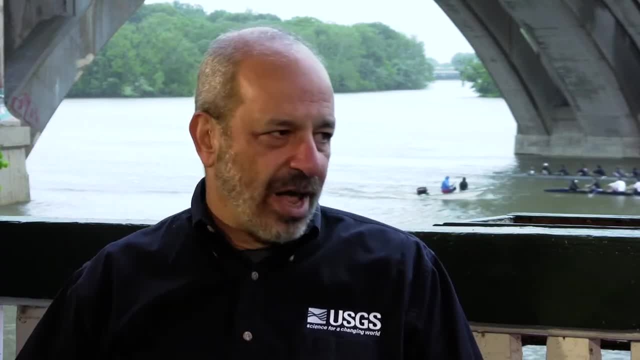 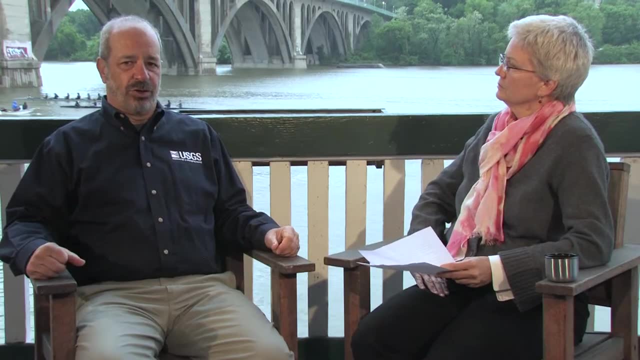 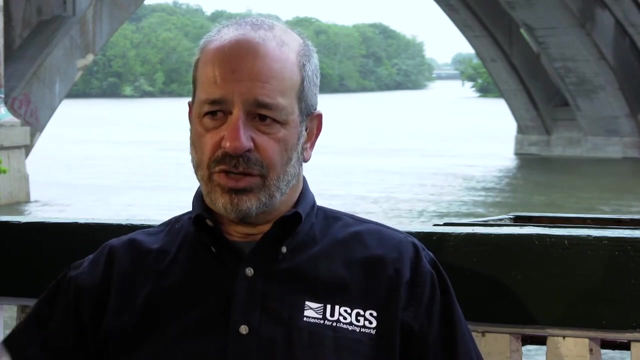 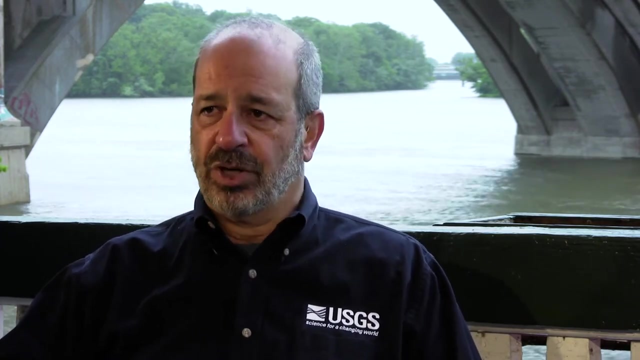 NAWQA works on a variety of scales, and each scale that it works at lends a possibility to answer certain kinds of questions. One of those scales is a very national scale, where we design and select monitoring locations of both rivers as well as groundwater, and measure a very consistent set of variables. 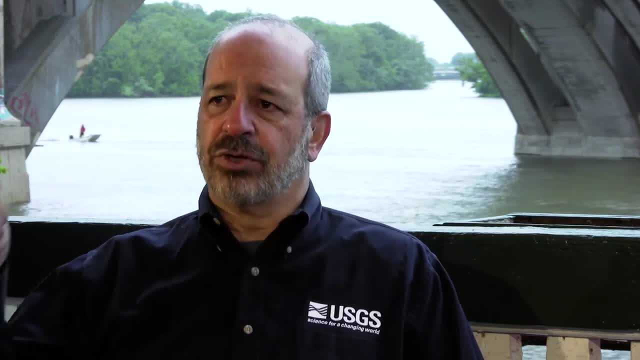 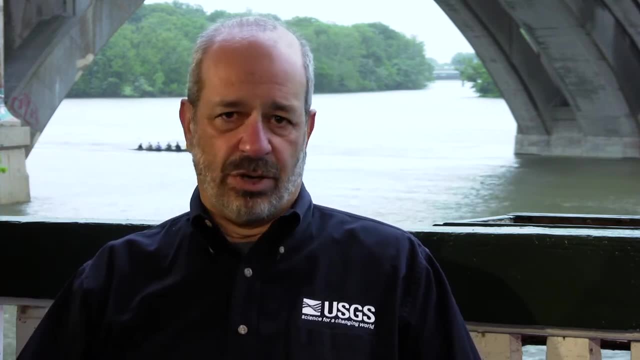 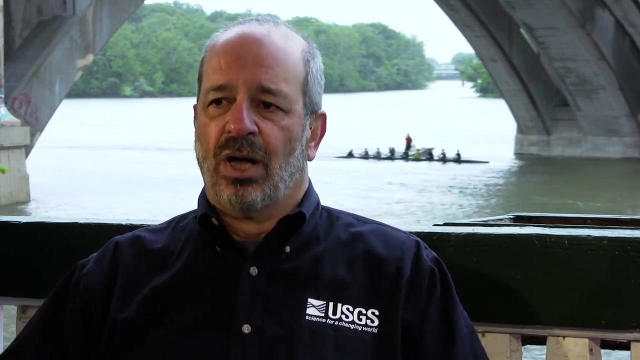 Things like the nutrients, nitrogen and phosphorus, the salts that are in the water, the man-made organic chemicals that are in the water and particularly the pesticides that are in the water, And we develop methodologies to measure those things on a wide network of sites. 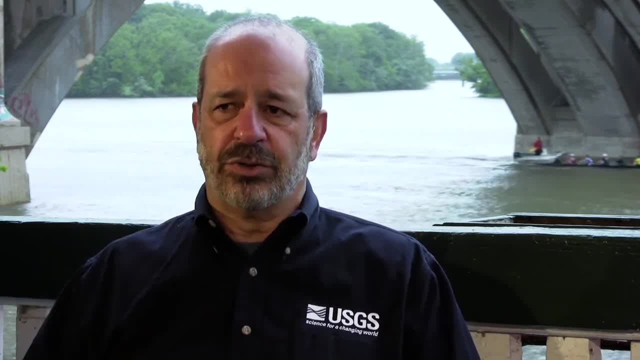 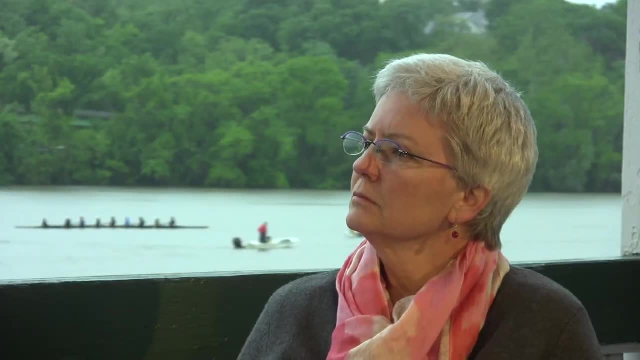 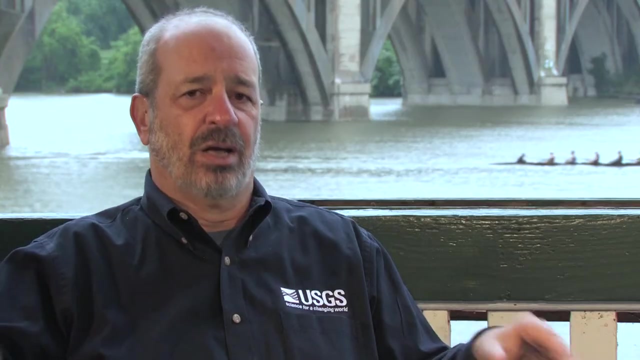 and we're able to say some things about what are the typical levels of those things in a wide variety of environments around the country, and develop statistical models that help us really fill in the mosaic of the waters of the nation and trying to understand, based on the geology, based on the climate, based on the land use. 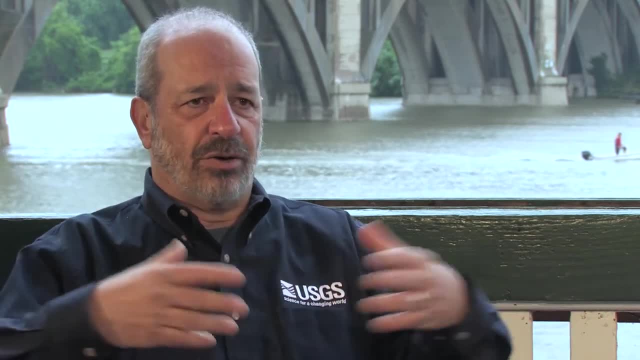 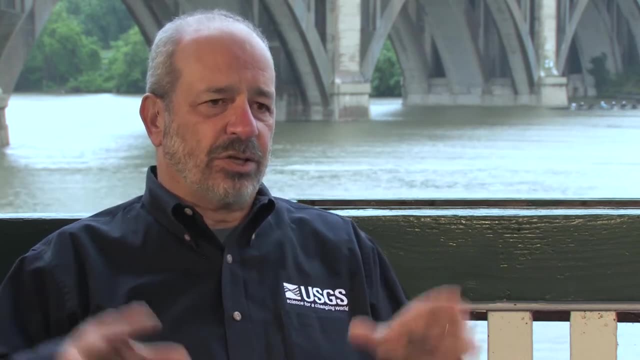 the population and the activities in that watershed or in that area, what kind of water quality is likely to be there, And that's a very important aspect. But at the same time, NAWQA has worked at the detailed scale, trying to understand processes and compare them across the country. 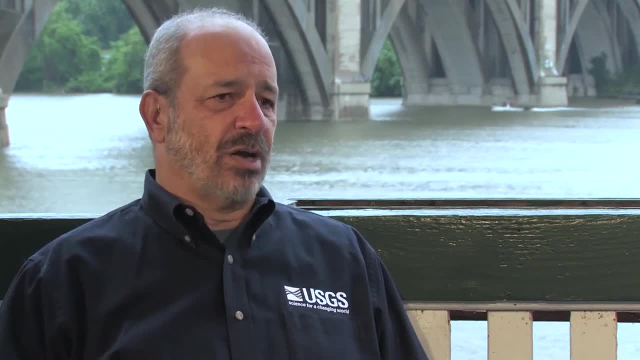 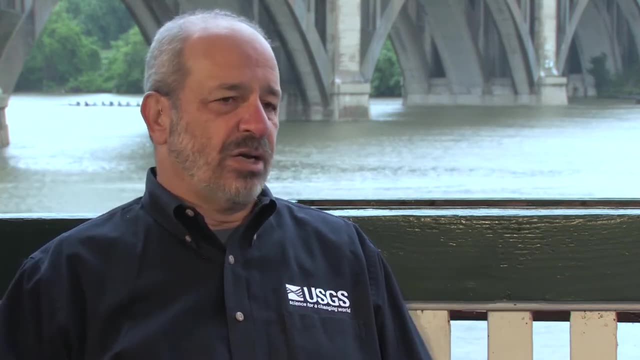 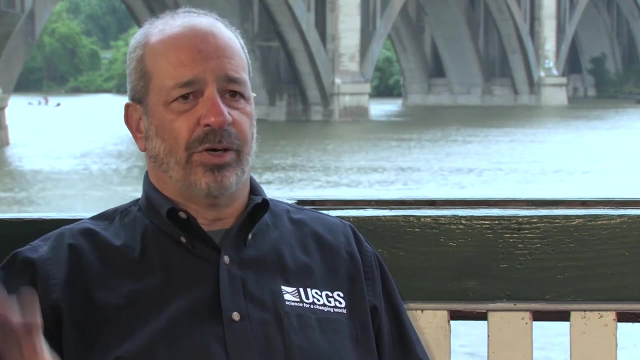 Across different areas. One of the best examples of that is our, I think, advancing the understanding of pollution from nitrate. Nitrate is a product of, particularly of fertilizers that are laid on the ground by farmers and by homeowners and by in urban areas. 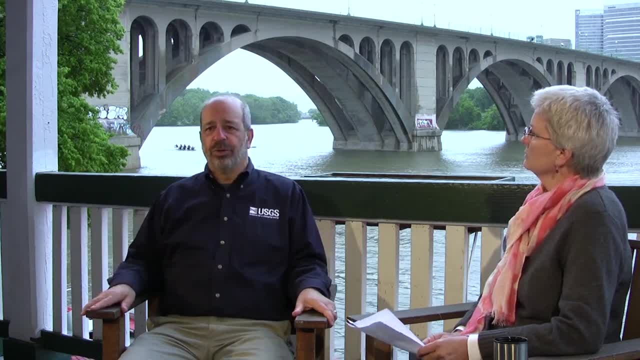 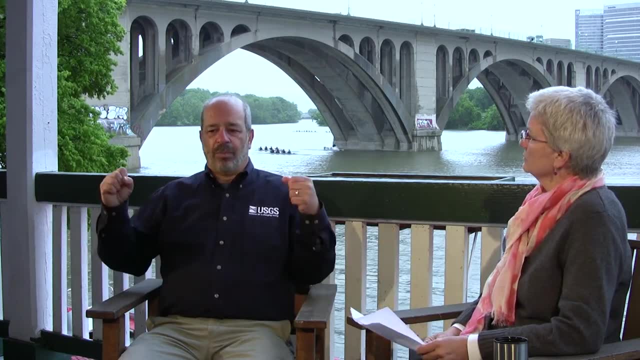 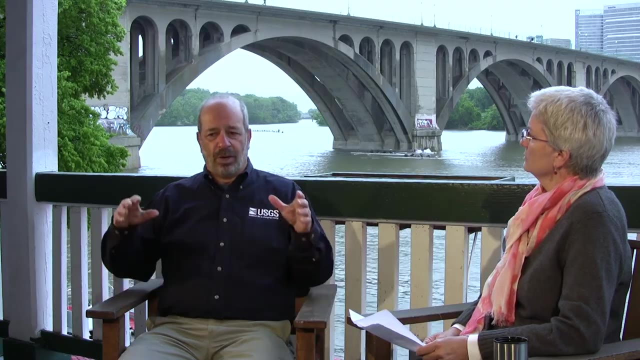 It also comes from the atmosphere, from the burning of fossil fuels, And it also comes from sewage. It comes from our wastes. Nitrate is harmful to humans if ingested. It's also an important pollutant to water bodies, causing algal populations to increase. 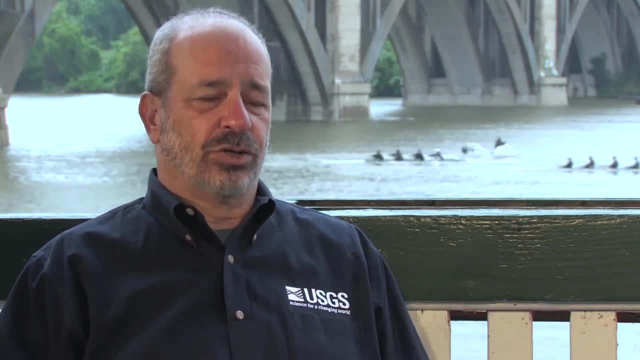 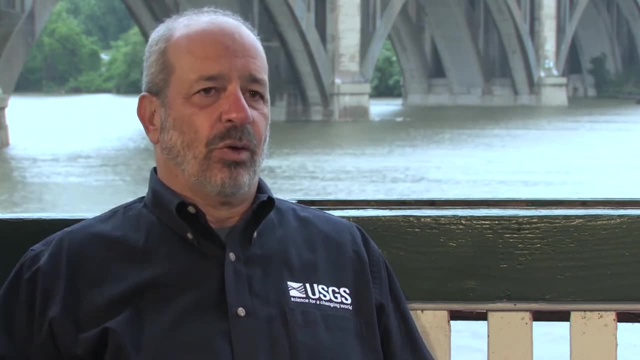 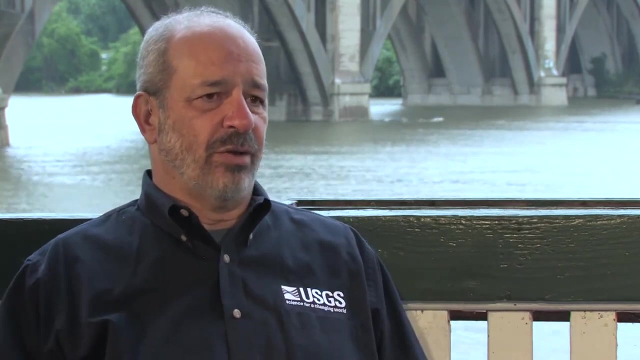 This process of eutrophication which is such a big concern in many parts of the country. In the NAWQA program in a wide variety of environments, we've been able to understand and describe what happens to nitrogen in those environments. 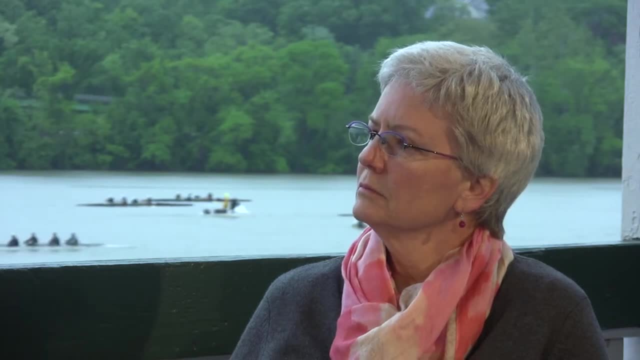 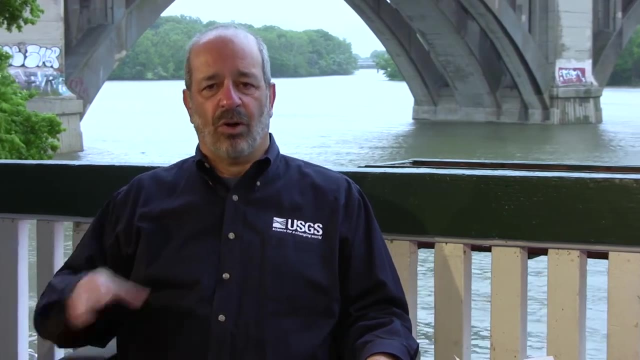 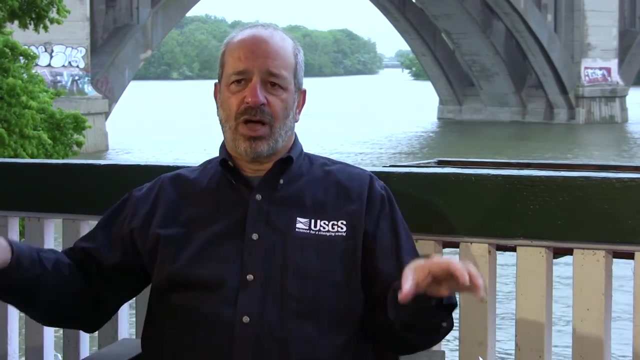 And in some cases there are natural purification processes, called denitrification, that clean up that before that water gets into the river or as it moves downstream In other areas. that doesn't happen And NAWQA using standard scientific protocols to understand those processes. 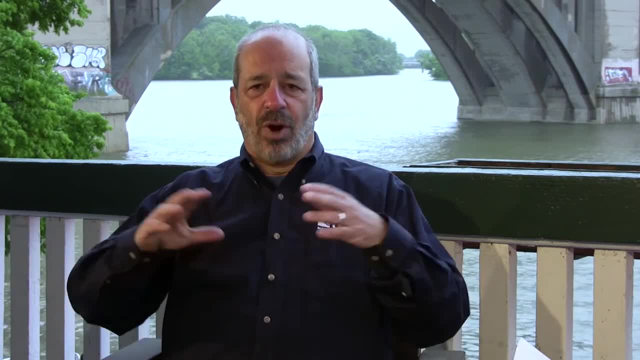 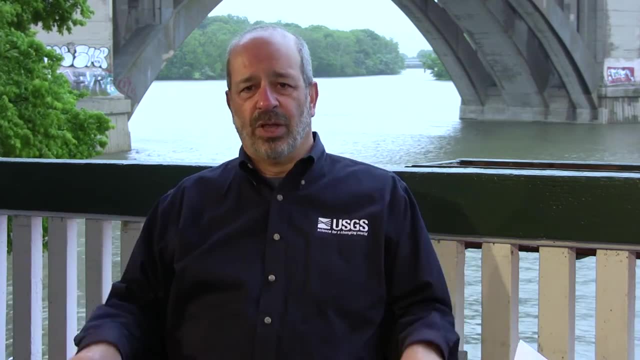 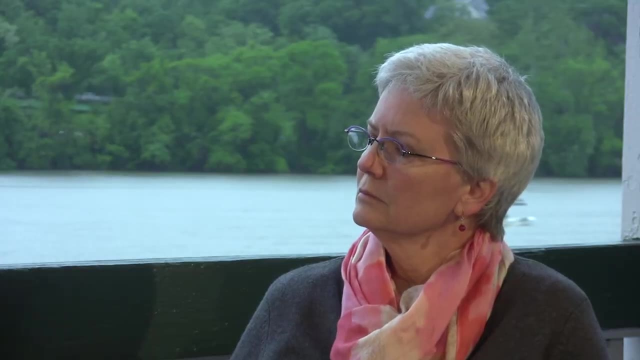 looking at a wide variety of areas has helped greatly in our understanding of where that natural purification works and where it doesn't work, And it gives us an ability to predict where those problems are going to exist and how, what it would take to reduce the extent of those problems.